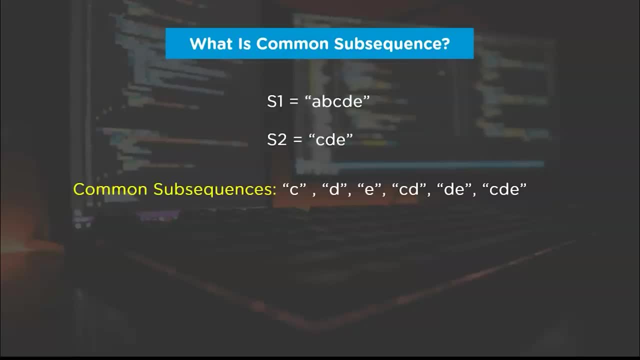 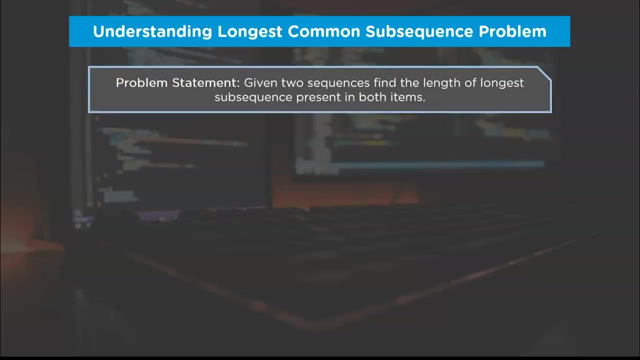 And from this you can clearly say that the longest common subsequence will be CDE Moving forward. let's dive further into this LCS problem to understand the logic behind The problem statement, for the LCS states that given two strings find the length of common subsequences present in both the strings. 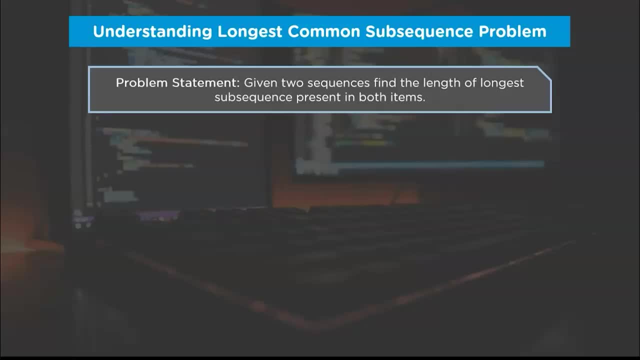 That means in this problem we'll be given two different strings, with length m and n respectively, And from these two strings we'll have to find the longest common subsequence with length k. Let's consider these two strings present on our screens. 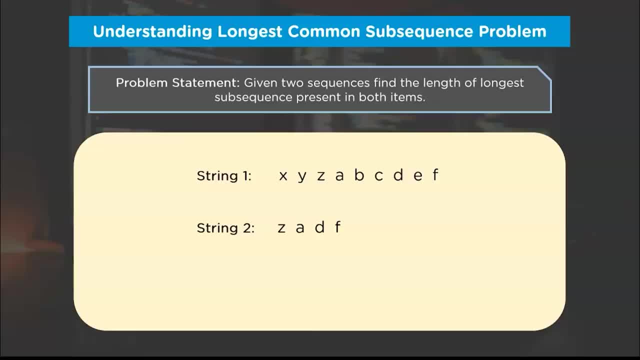 We'll try to find out the LCS for both of these strings. here We'll try to map patterns present in string 2 to string 1.. Now let's pick the first character in string 2, ie z. Now we'll match this character to the character present in string 1.. 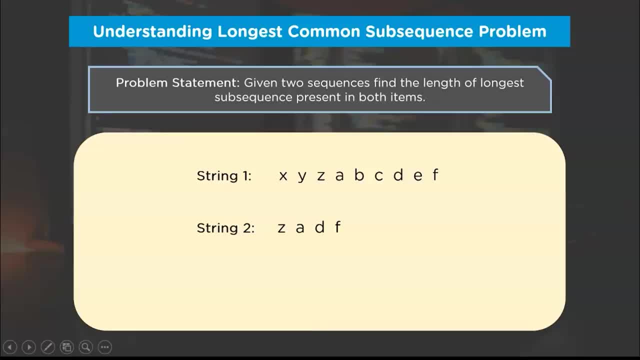 And the first character is x, So we'll map it with x, But z and x do not match, Hence we'll move towards the next character. Next character is y And z, and y also does not match Hence we'll move to the third character, ie z. 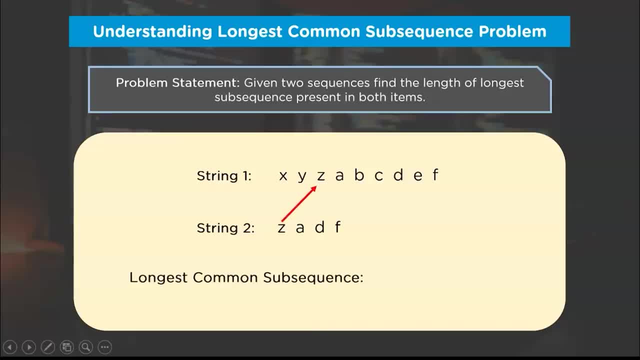 Here we have found the match, So what we'll do is we'll include z into our longest common subsequence. The next character in our sequence is a, And we have a in string 1 as well. Hence we'll include a in our longest common subsequence. 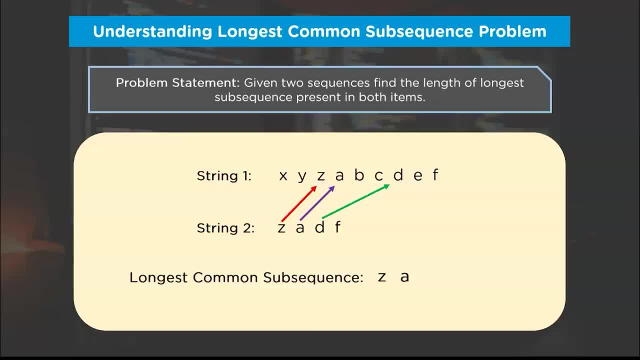 The next character in string 2 is d, And we have found match for d in string 1 as well, Hence we'll include it in our longest common subsequence. The final character in string 2 is f, And we have found f in string 1 as well. 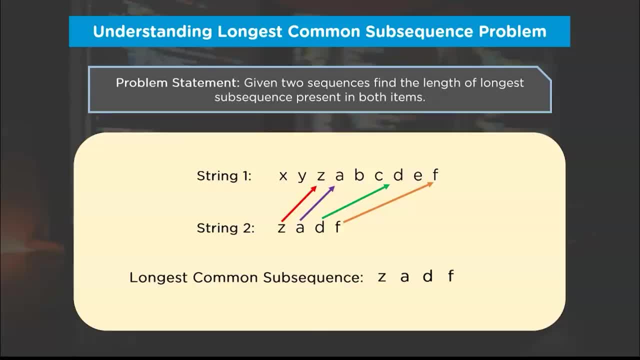 Hence we'll also include it in our longest common subsequence. Finally, the longest common subsequence for string 1 and string 2 will be z, a, d, f, Moving forward. let's discuss one more problem to understand LCS clearly. 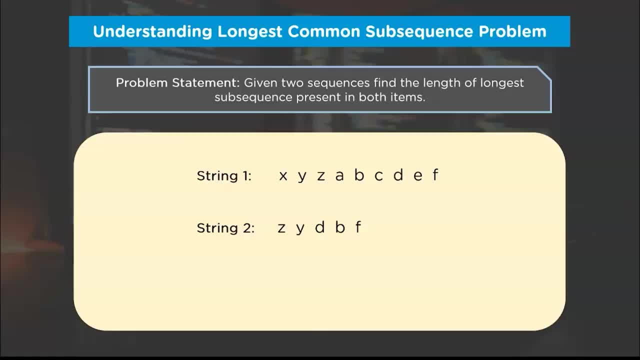 Here you can see that z is present in both the strings. Thus we'll include it in our LCS change. The next character is y. It is also present in string 1. But the rule of LCS says that the sequence of character should not be changed. 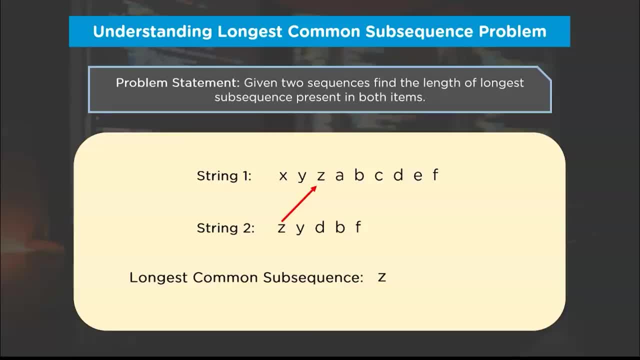 And here the mapping line of z and y are intersecting. So we'll discard character y here And we'll pick the next character in string 2.. That character is d, And d is not intersecting with any other character. 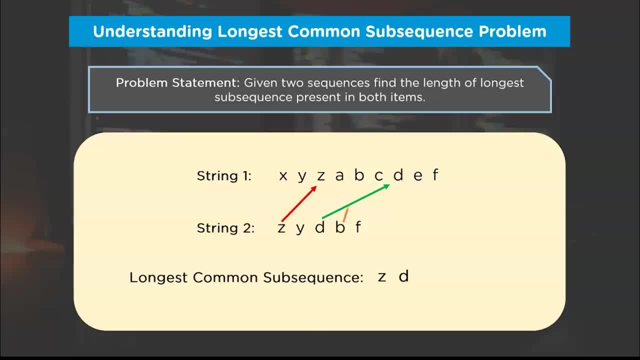 Hence we'll add it to our LCS string. Now the next character b is also there in string 1.. But we cannot insert it in our LCS string as it intersects with the mapping line of character d. Thus we'll discard this character. 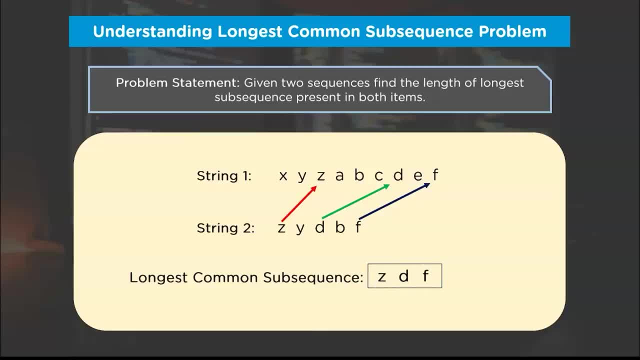 The next character f can be added to our LCS string as it does not intersect with any other mapping line. So the first LCS sequence will be z, d, f And, due to multiple intersections, there is possibility of having another sequence that can be larger in length than the previous sequence. 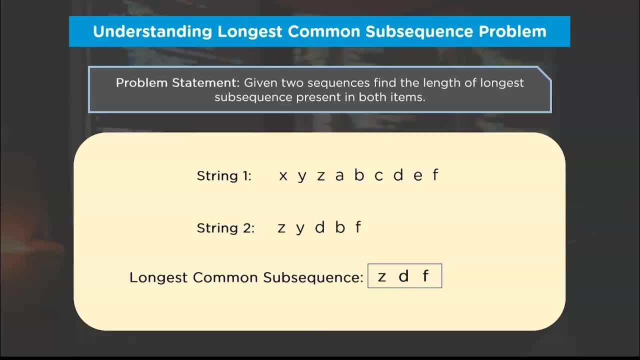 For this sequence we'll begin from the second character of string 2.. That is y, And y is present in string 1.. Thus we can add it to the LCS. Next we can add d to our LCS sequence. After this we have b. 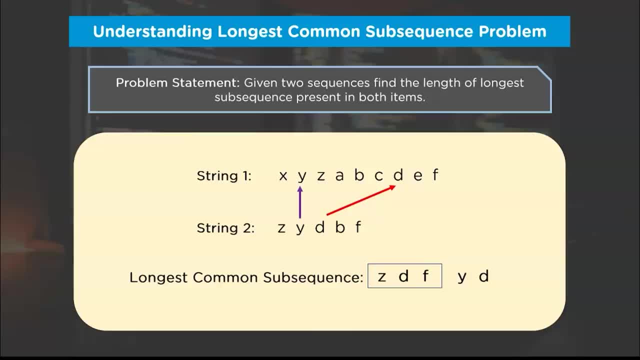 But b cannot be inserted into LCS as it is intersecting with d, Hence we'll discard it. And finally we'll include f into our LCS sequence. In this problem, both the sequences have the same length, Hence both of these sequences will be considered as Longest Common Subsequences. 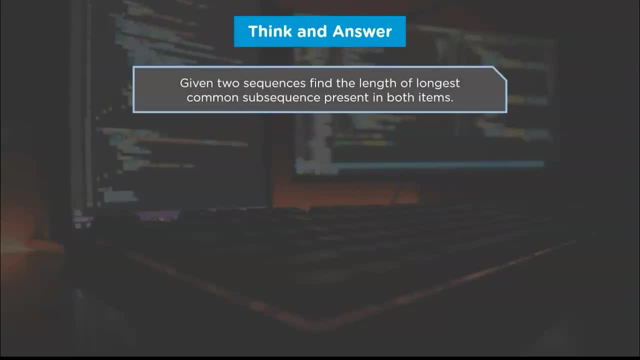 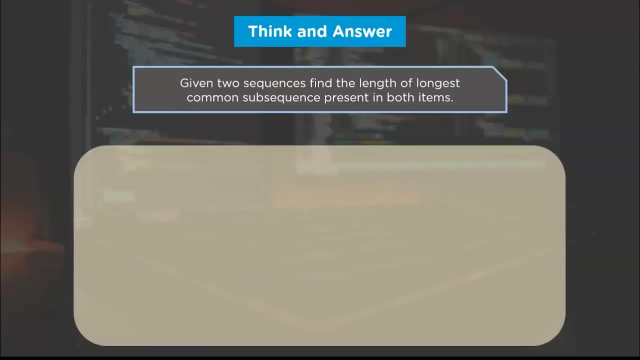 I hope that you guys have understood the logic behind finding the Longest Common Subsequence, Cause we have a challenge for you guys to assess your understanding of the LCS. For these given sequences, you're supposed to find out the Longest Common Subsequence. 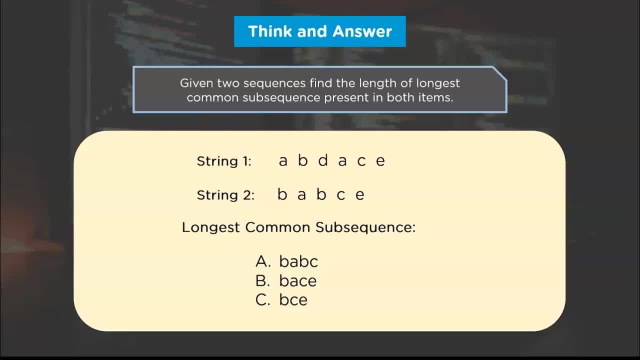 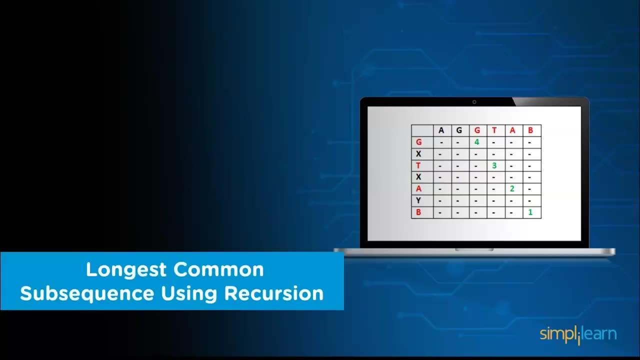 The options for this problem are b-a-b-c, b-a-c-e and b-c-e. You all can drop your answers in the comment box below. Let's see how many of us can get this right Now. moving forward, we'll build a solution for LCS using recursion. So let's visit the code editor and develop the C program for Longest Common Subsequence. The two strings for which we are going to find LCS are xy and xb. Let's create a function to get started with LCS implementation. I'm going to name this function as int lcs. 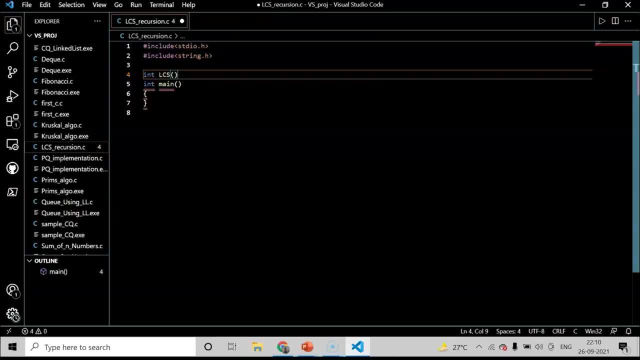 And inside this function we'll pass the references of two character edits. The first will be char star a, comma, char star b. The next arguments will be the links of these character arrays: int x and int y. Now we'll move to the function body of LCS. 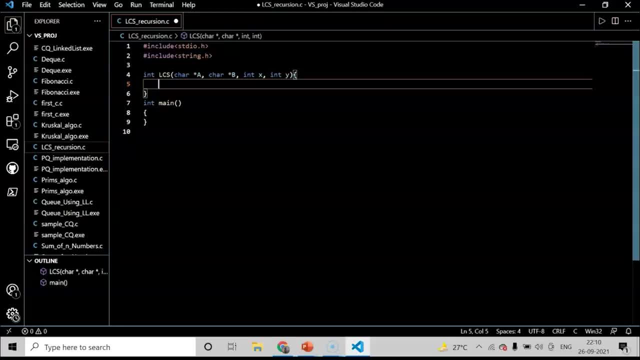 The first condition we'll evaluate is if the character arrays are empty or not, Because if character arrays are empty, then definitely there won't be any sequence to find out. So when we reach x equal to 0 and y is equal to 0, we'll return 0.. 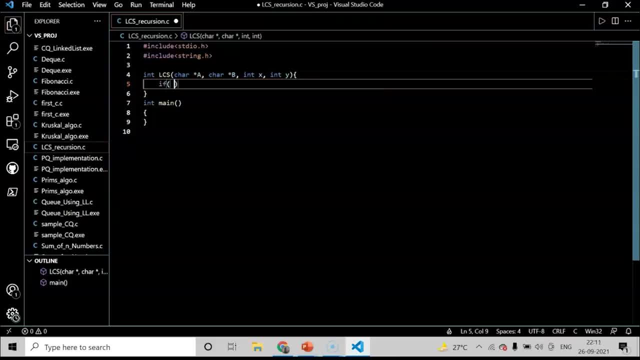 For that we'll write a condition: if x equal to equal to 0 or y equal to equal to 0, then return 0.. Now the next condition: when both x and y won't be 0, we'll check if the last character of both character arrays match or not. 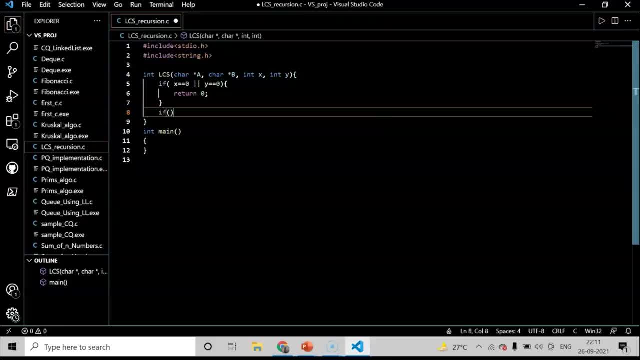 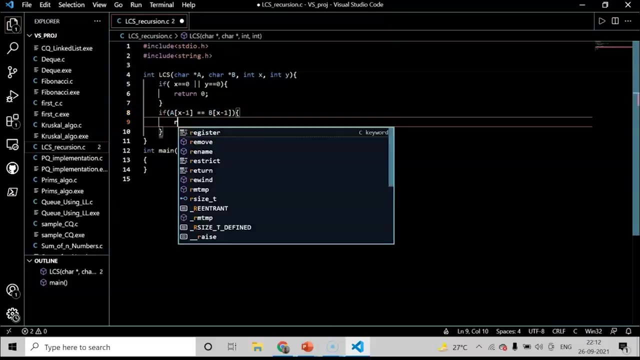 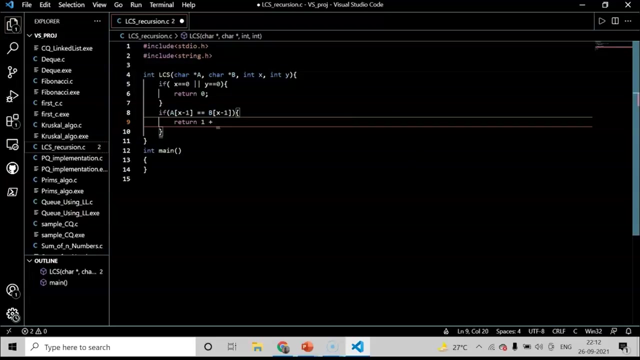 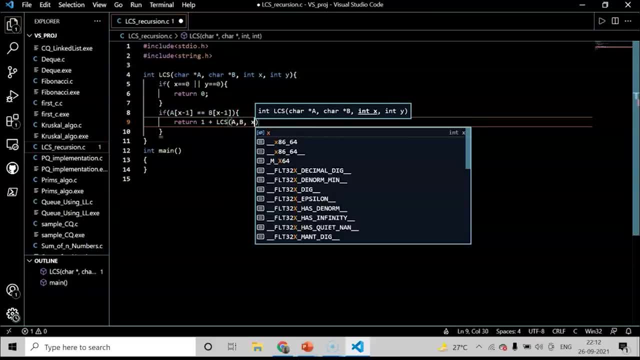 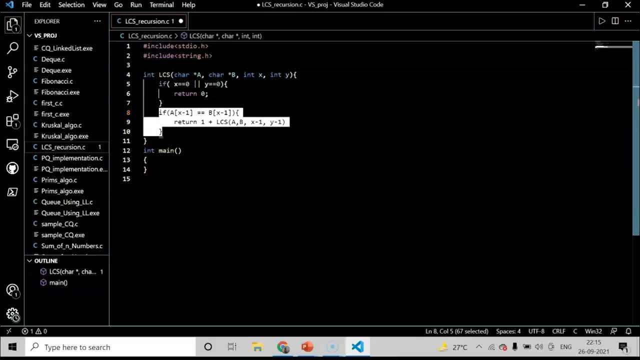 Then we'll return 1 plus LCS. Then we'll return 1 plus LCS. Then we'll return 1 plus LCS Once this condition gets fulfilled, 1 plus recursive call to LCS. function With inputs decrease in size by 1, ie, x minus 1 and y minus 1.. 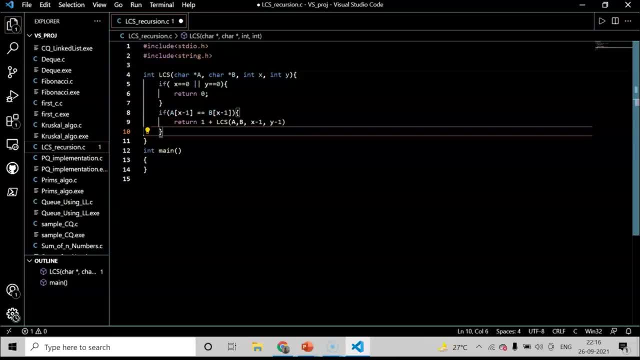 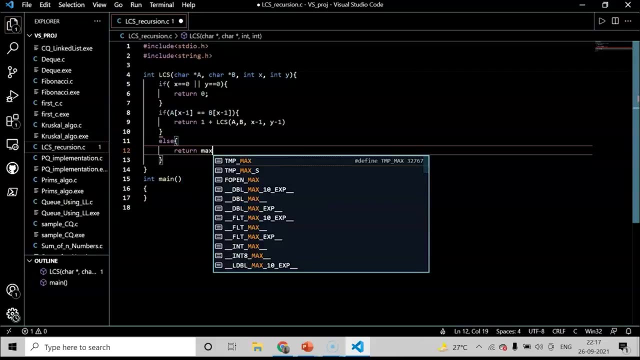 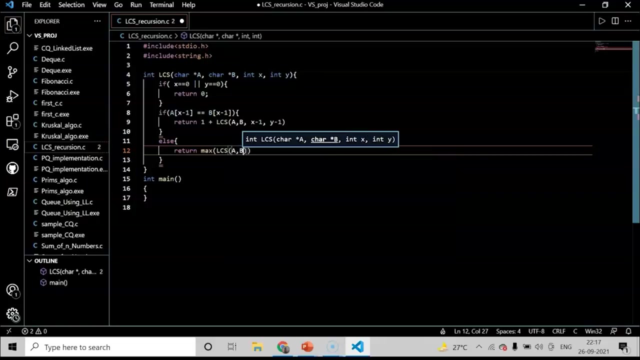 1 plus recursive call to LCS function. Now, if both the previous conditions fail, Then we'll enter unsuzailable. so'll write some ins quems And insesco: siinde li beh albe, We will return max of LCS or LCS a comma b, comma x minus 1 comma y. 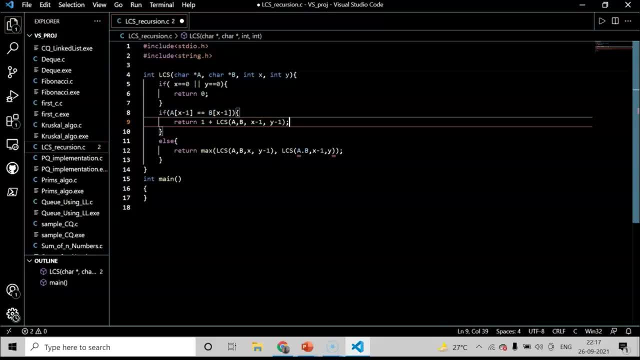 We are missing semicolon here, Okay, and dot here, So we will change it Now. this statement, This statement will get executed when there is no character match. If characters don't match, we will move either way: one character in first string a or one character in second string b. 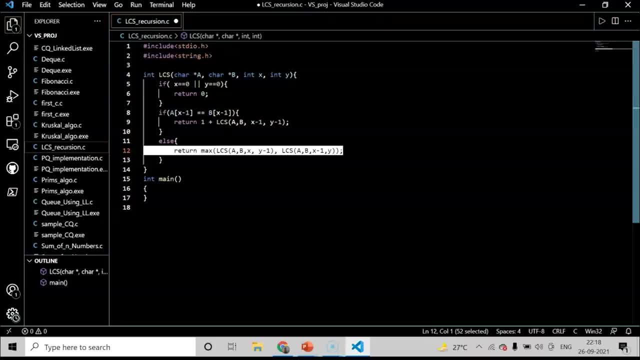 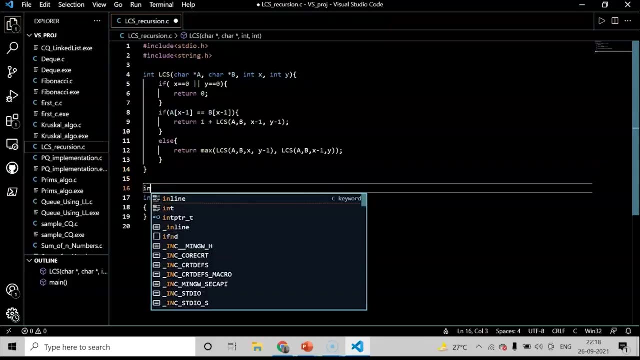 and check whichever gives maximum, and we will take that into consideration Most of the time this condition will get satisfied. To find out the maximum we will have to create a manual maximum function. So for that we will create a new function that is int max. 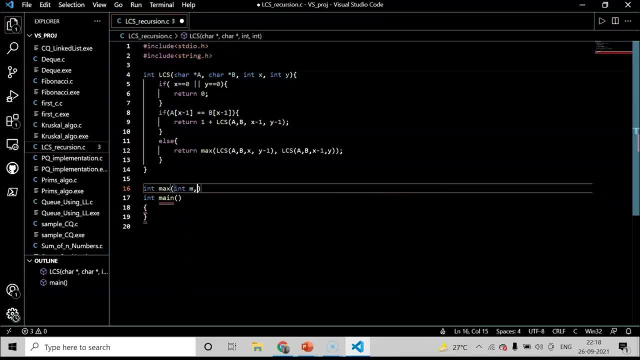 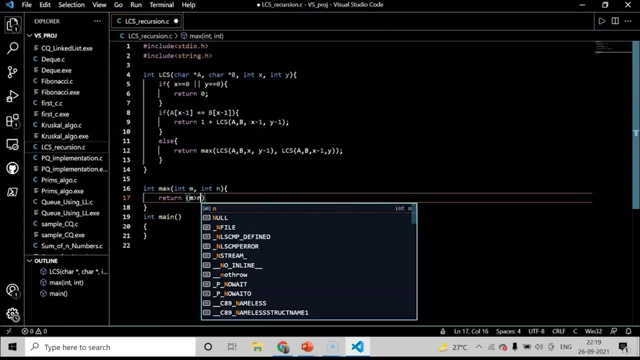 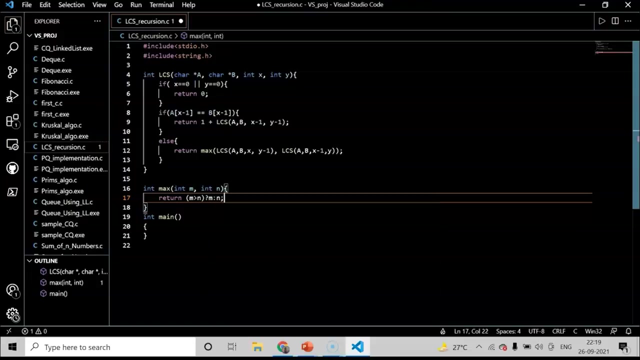 And we will pass arguments: int, m, comma, int n. Now, inside this function we will write a ternary condition that is return m greater than n, question mark, m, colon, n, semicolon. So this will return the maximum value between m or n. 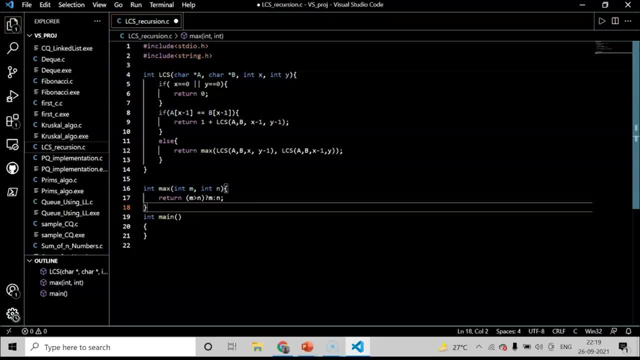 With this we have successfully completed the LCS function. So, moving forward, let's work on our driver function. In driver function, what we will do is we will create two character arrays at first. So for that let's enter into this main function and we will create character array a, and inside a we will pass x and y. 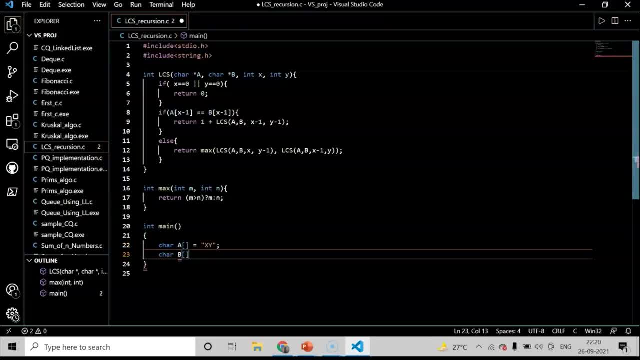 We will pass x, b, y, q And we will store the lengths of these character arrays into x and y. For int x is equal to str len a And for int y, strlen b. We will add semicolons here And finally we will make call to our lcs function. 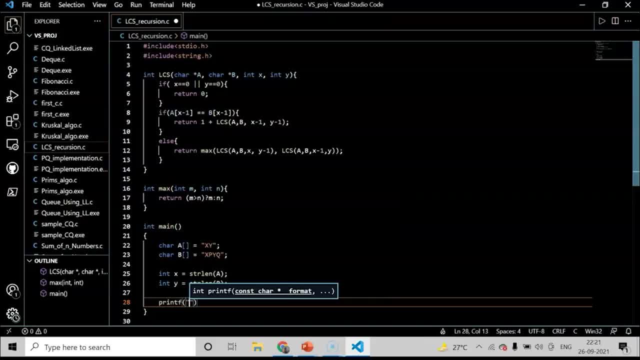 using the printf statement. The printf statement that we will write is: link of lcs, is modulus d comma lcs, a comma b comma, x comma y semicolon, And finally, we will add return 0.. I hope our code is bug free now, So let's run it. 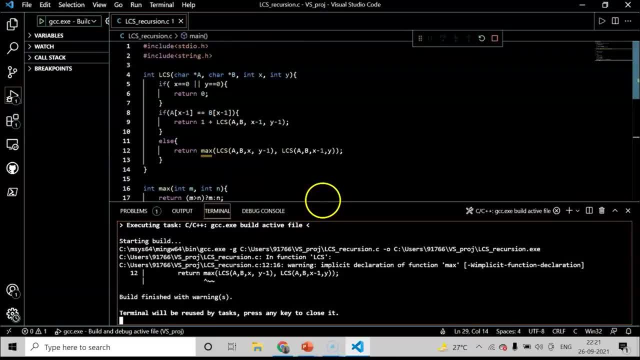 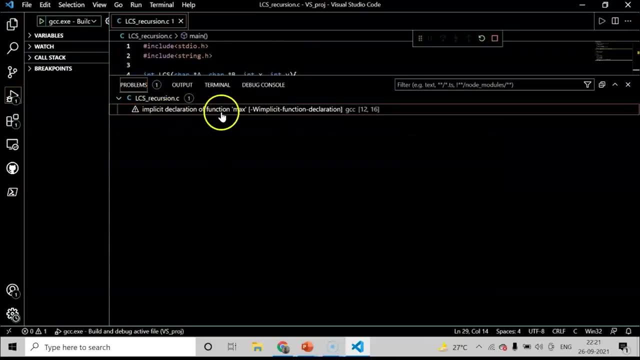 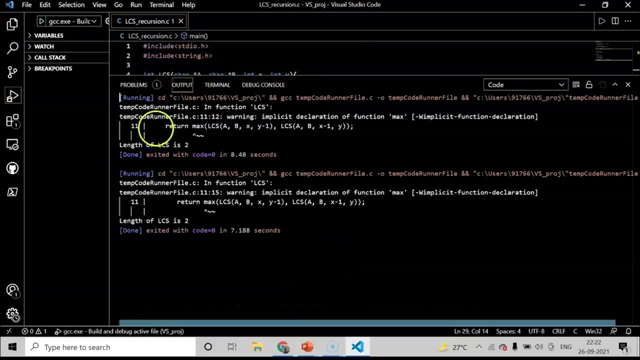 And check if it is bug free. That's fine. Here we are getting error, but it is not exactly an error. We have implicitly declared function max here, So that's why we are getting this flag problem, But we are actually getting output as well. So 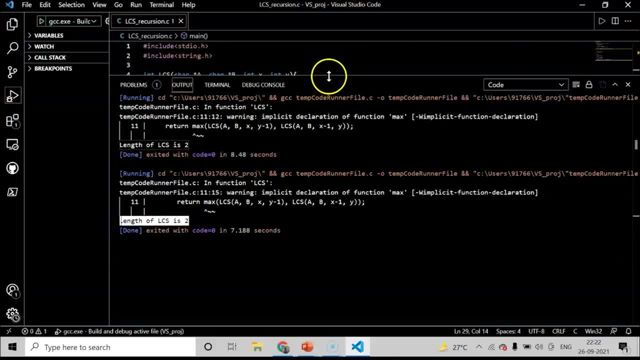 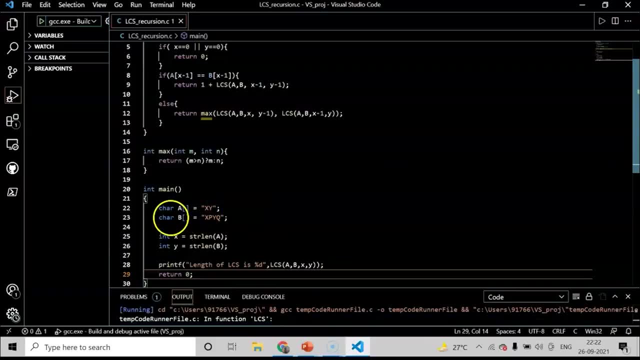 the output that we are getting is two here, And if you check both the strings, then you can find out that character array a is implemented inside character array b And the length of common sequence is two here. So with this we can say that our recursive implementation of lcs is successful. 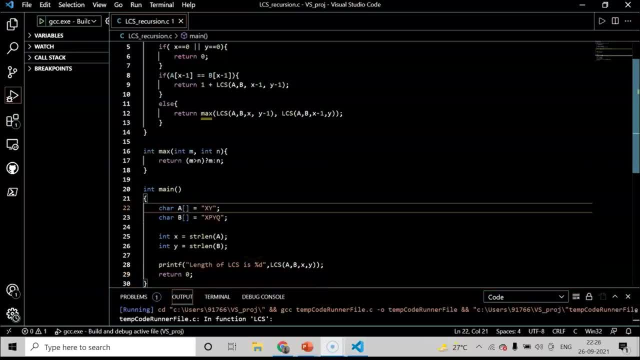 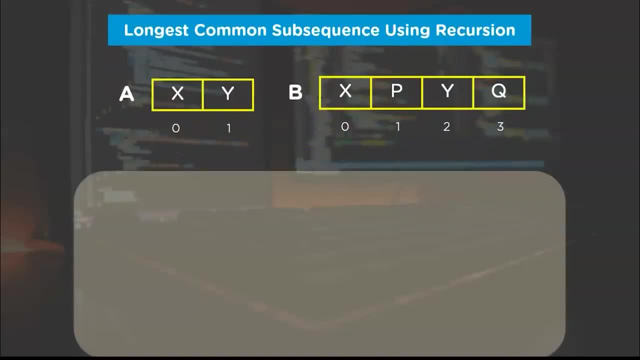 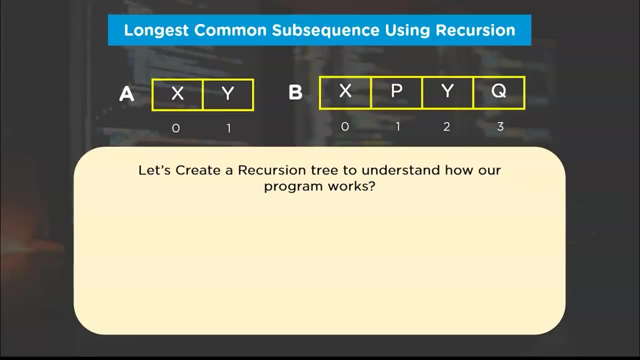 Now moving forward. we'll visit PowerPoint to understand why recursion is not an ideal approach to solve this problem. To understand the complexities associated with longest common subsequence problem implementation using recursion, we'll formulate a recursive tree by going through the steps of a program. 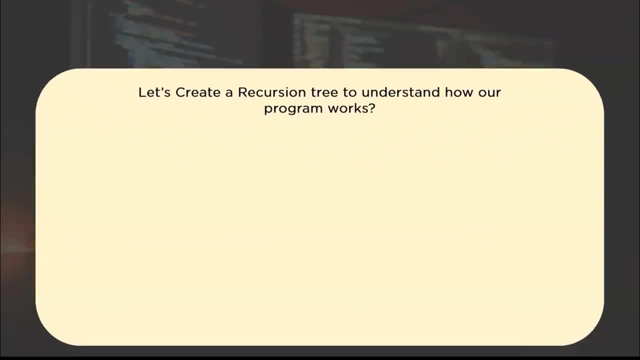 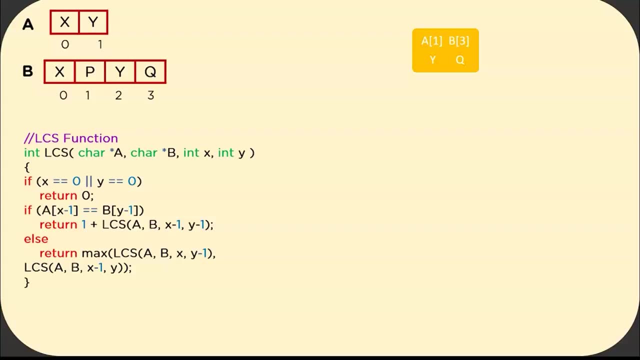 that we have created previously, So let's do that here. As you can see, in this lcs function, the first step we perform is checking if both the strings are empty. If they are not empty, then we check if the last character of both strings matches or. 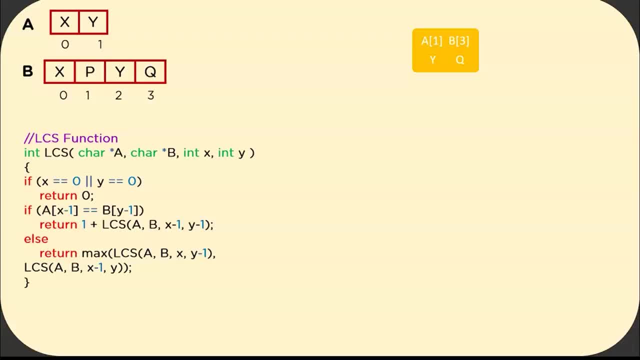 not. Thus, the first call to the lcs function will check for the match of last two characters. If characters don't match, which is true in this scenario, we move either one character in string a or in second string b, And we'll choose whichever produces maximum value. 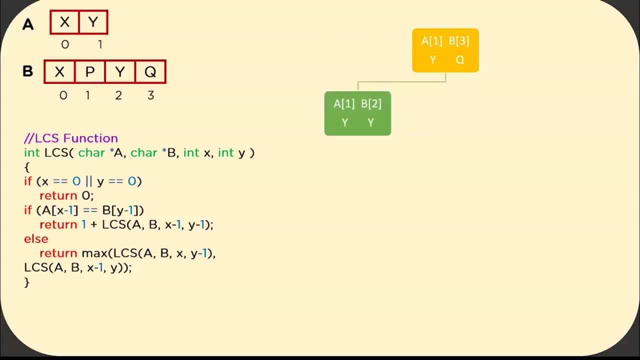 So if we reduce b by one and keep the a same, then we have a character y in both the strings, Whereas if we keep b the same and reduce a by 1, then we have x and q which don't match with each other. 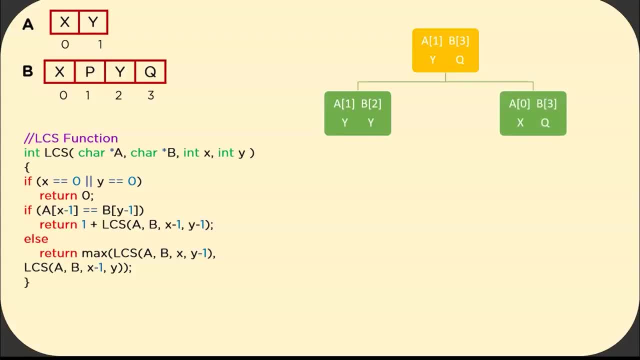 First we will evaluate the left side of our recursion tree and here we have a character match. thus we will enter if condition where characters do match. that is this condition and it says that return 1 plus both the character arrays with size reduced by 1 and by doing: 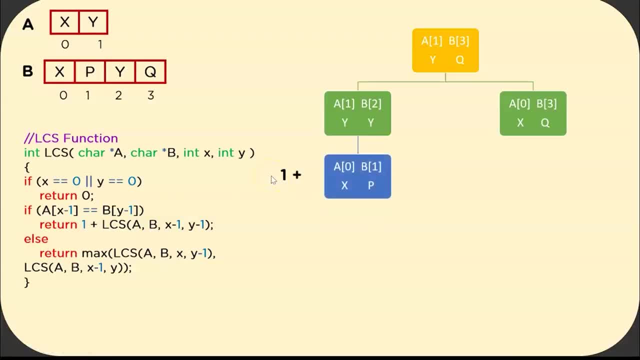 that we get two different characters, x and p, here. Now, as these characters do not match, we will move position by 1 in both the strings. by doing that we get these results and here, if we observe, the left child has a character match. thus we will add 1 and reduce the size of both character arrays by 1, and with this 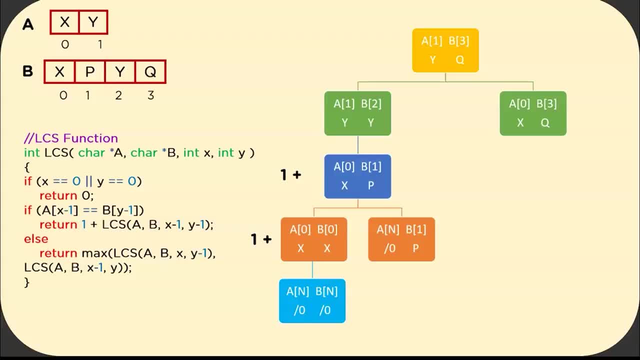 step we reach the end of our strings. Now let's work on the right side of our recursion tree. In this case we have distribution. We have two distinct characters. thus we will move by 1 in both. the character arrays and the resultant child nodes don't have characters that match. 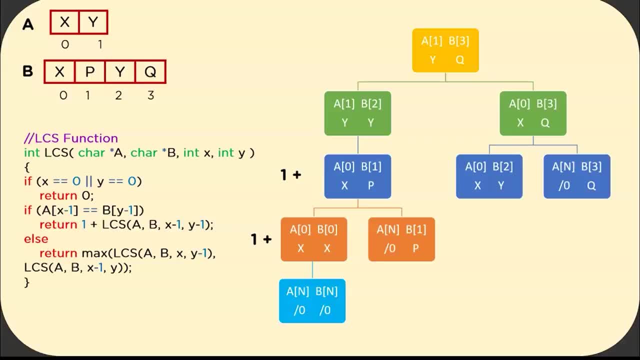 Furthermore, the right child reaches the null index. hence now we will just expand the left child. In addition to that, we can move positions only in character array b, as we have reached the end of character array a. For this move we do not have any match, so we will reduce the position of b by 1 again. 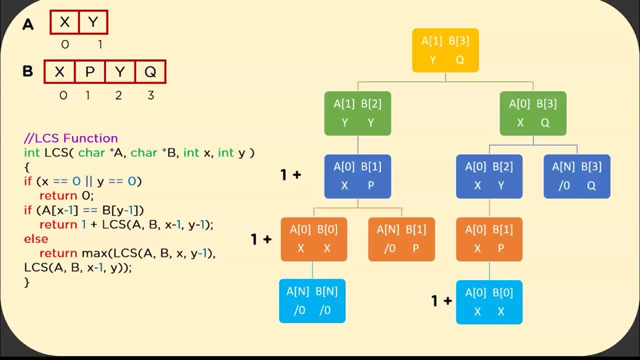 And here we get a match And also reach the end of both character arrays. Now the next step will be for evaluating LCS length by backtracking our recursive tree. First we will consider the left side, so let's begin from the bottom of left side. 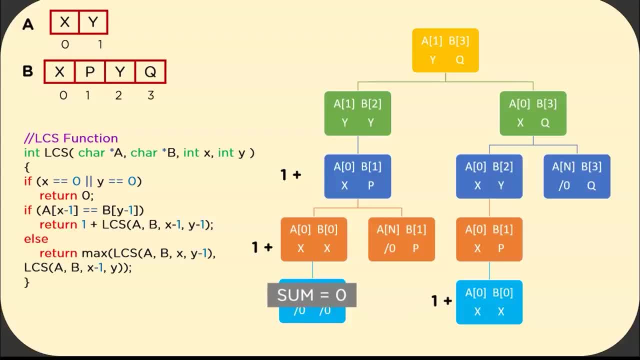 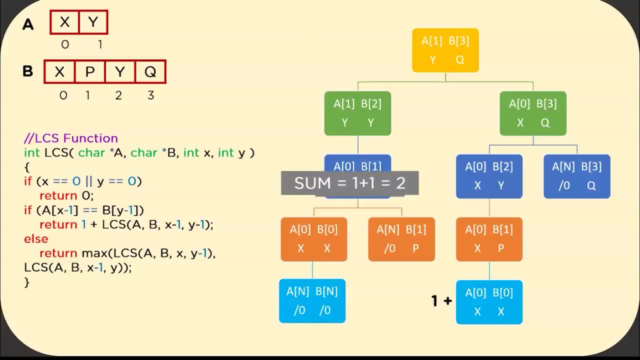 Thus the sum value will become 2 here And the overall sum for the left side of recursive tree will result into 2.. Whereas for right side the sum will become 1, as there is only one match Now. this side, which has maximum sum value, will be returned as a result of this LCS program. 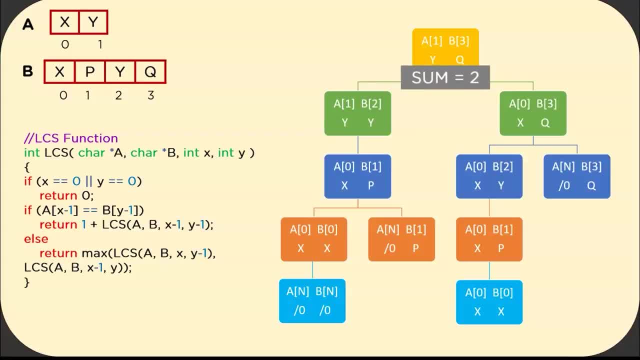 which will be 2. in this case, The complexity for this recursive LCS program will be 2.. Now for these two strings which have small length. you can see that the complexity will be equal to 2. to the power n where n belongs to the depth of binary tree. 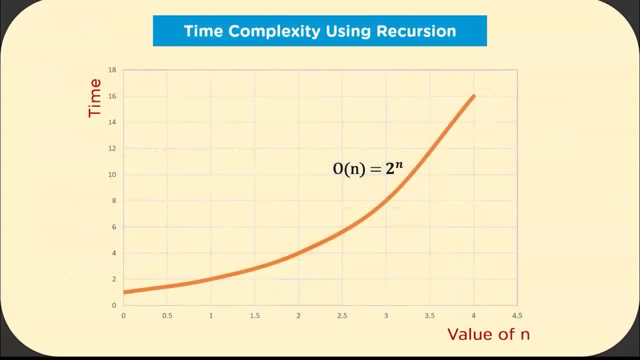 That is huge complexity. If you look at the complexity graph, you will get that. you will get parabolic graph which will increase continuously or exponentially. However, this problem can be resolved by using dynamic programming paradigm. Moving further, we will talk about the dynamic programming paradigm. 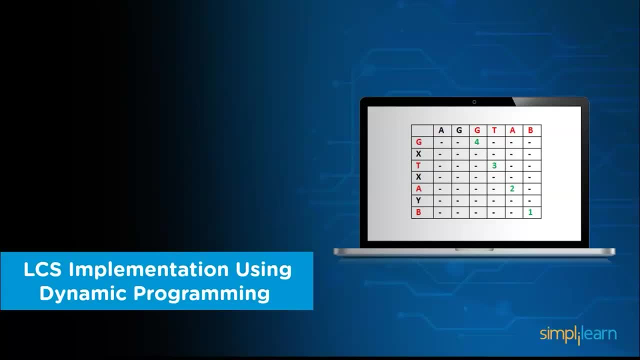 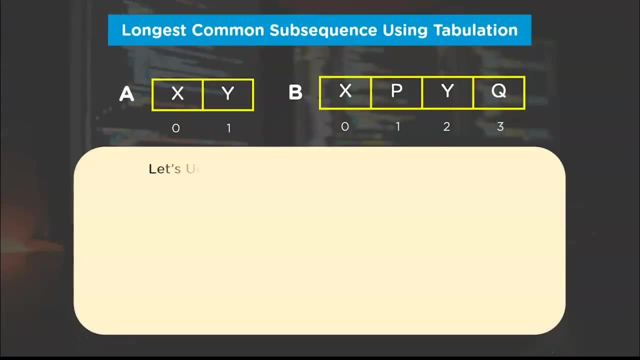 Moving further, we will talk about the dynamic programming paradigm. We will try to analyze how dynamic programming can reduce the computational complexity of LCS problem. Here we will try to solve LCS problem using the tabulation method in order to understand how tabulation can reduce space complexity by making fewer computations. 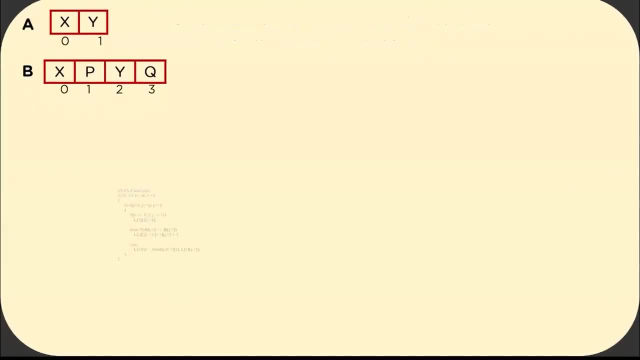 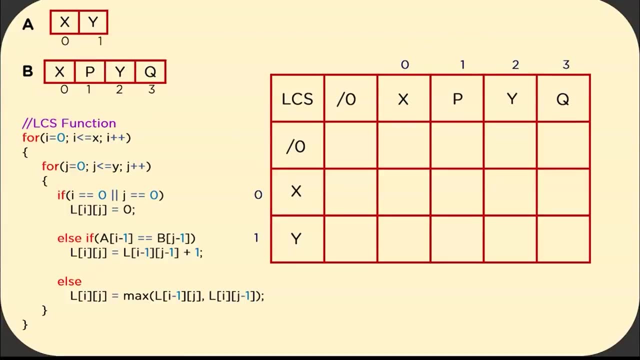 The LCS function for tabulation will be iterative, Hence we will understand the computation with the help of tabular representation. The columns will represent character array B. Furthermore, we have added the null values to the table, Hence initially we will set the field values for null row and columns as 0.. 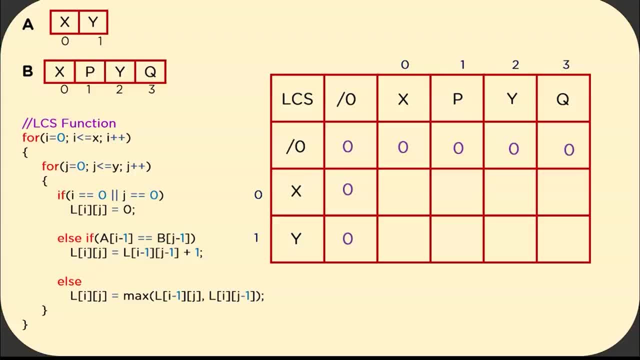 Now here we will move through the row of character x. For the first iteration, we hit the match, Hence we will add 1 to the diagonal element, So 0 plus 1 will become 1.. For the next iteration, we get x and p, which do not match. 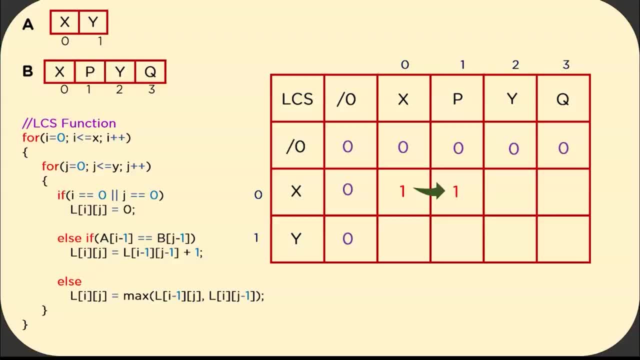 Hence we will add 1 to the diagonal element, So 0 plus 1 will become 1.. Hence we will add 1 to the diagonal element, So 0 plus 1 will become 1.. So 0 plus 1 will become 1.. 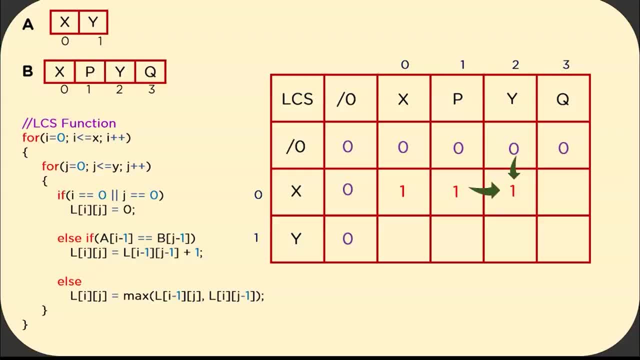 Next we have x and y, which also do not match. Hence we will continue with 1.. Remember, guys, the highest value between these two fields will be picked every time For the next move. the value 1 will continue. Now, moving forward, we will move towards the y row. 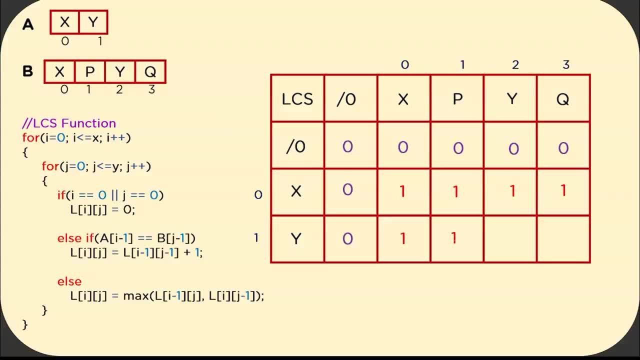 Here, for both x and p, the values will remain 1, as we don't have the character match. But for the next field we will hit the match. So 0 plus 1 will become 1.. So 0 plus 1 will become 1.. 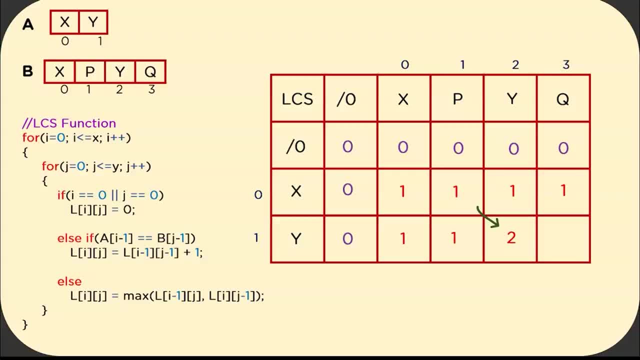 Hence we will add 1 to the diagonal field. The value for this particular field will become 2. now For the last field. the value 2 will get continued, as it is the highest field than the another comparative field, And you can see that we have found the accurate result here, which is 2.. 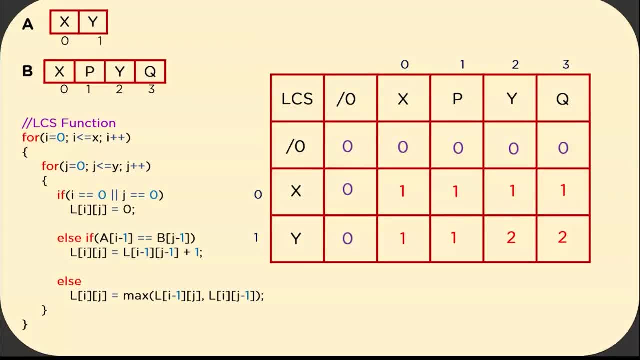 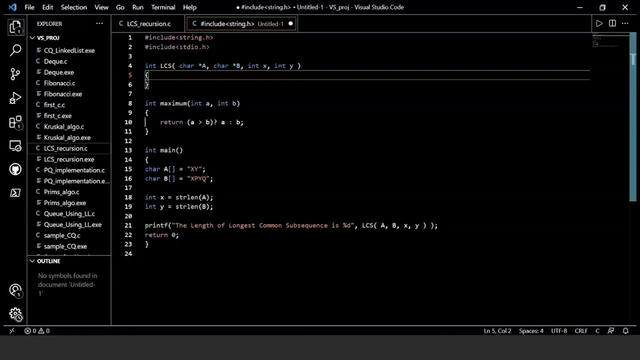 I hope this tabulation logic is clear to all of you, Cause, moving forward, we will develop a C program for the same. Now, in order to get started with this tabulation function, we have created intLCS function with few arguments. These arguments are similar. 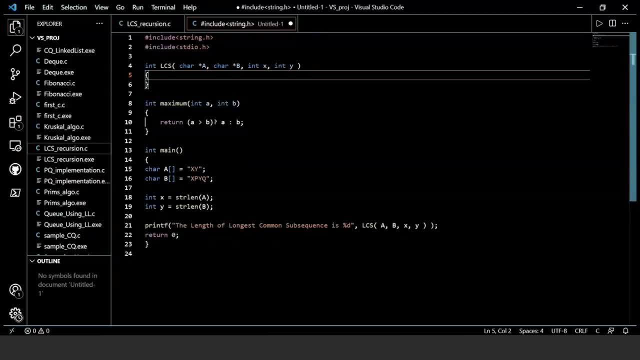 to the recursion In this tabulationLCS function, we will first create the 2D matrix for performing the computation. The statement that will help to do that is int L, x plus 1, x plus 1 and y plus 1.. 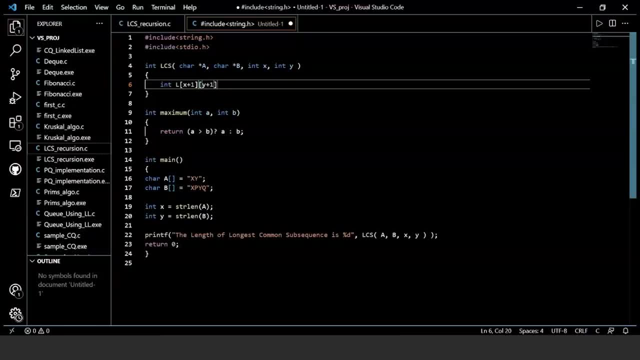 So this will create a 2D matrix of size x and y. We will also initialize few variables for using them inside looping process. So I will create a 2D matrix of size x and y. We will also initialize a few variables for using them inside looping process. 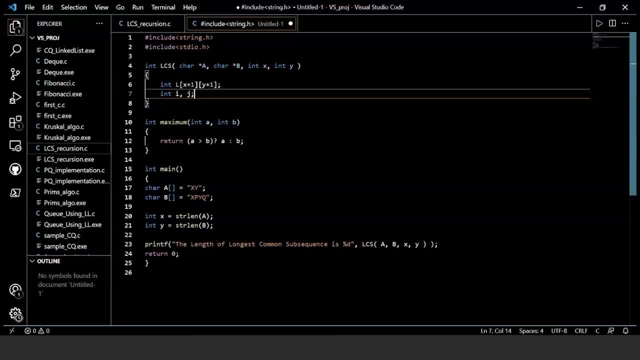 So I will initialize a few variables for using them inside looping process. So I will initialize two variables: int i and j. Next we will create a nested loops for traversing through both arrays at the same time and updating the computational table. For that we will create for loop and 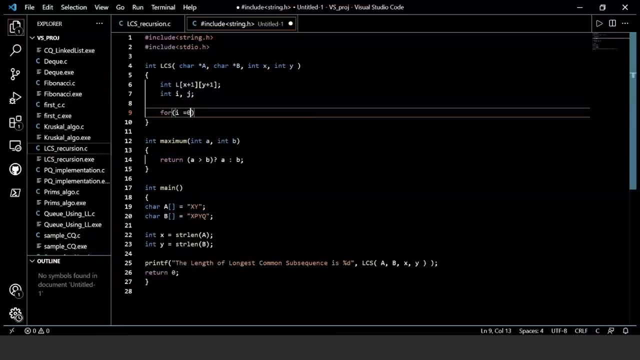 inside this for loop, we will begin from: i is equal to 0 to i is greater than equal to x, and we will increment the i And inside this for we will create another for loop and we will begin this with: j is equal to 0 to j less than or equal to y and j plus plus. 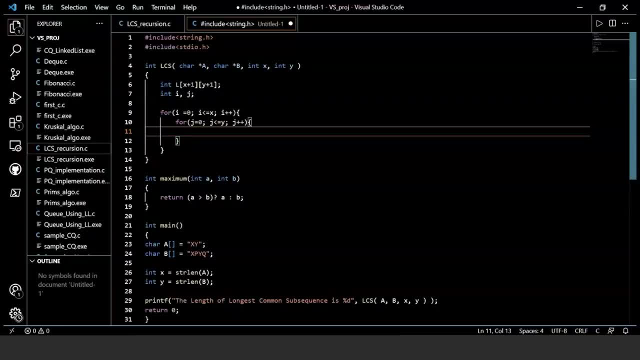 After that we will write the first condition to set null values for the null row and column fields. So the statement that we will write is: if i is equal to equal to 0 or j is equal to equal to 0, then set L i. 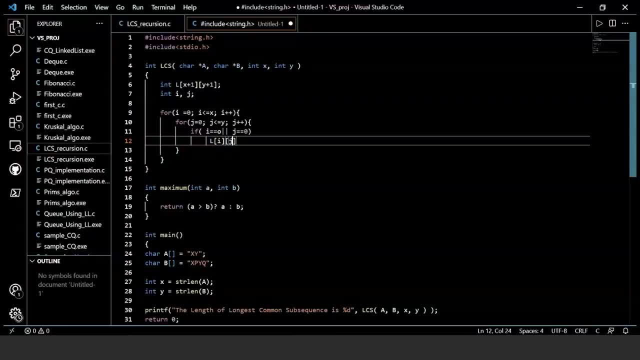 i j equal to 0.. If this condition fails, then we will check if the last character match with one another. If they match, then we will return 1 plus both array fields reduced by position 1.. For that we will write condition else if 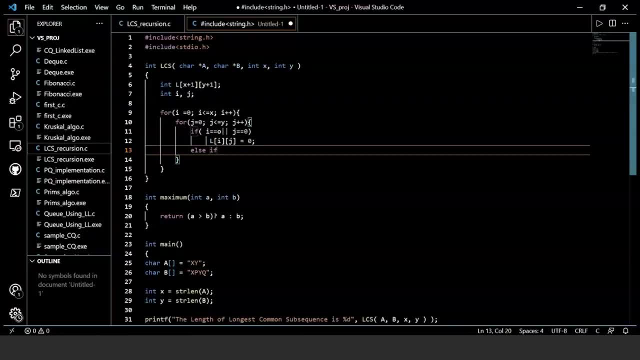 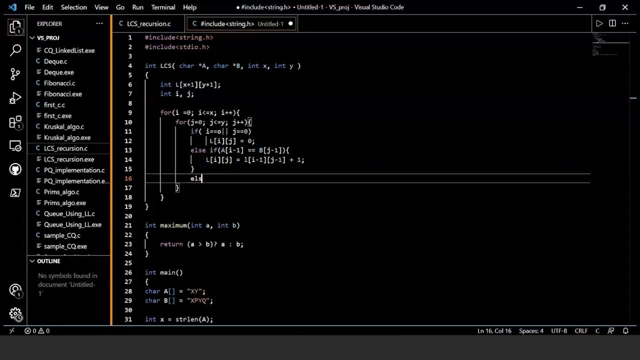 else, if a- i, i minus 1 equal to equal to b j minus 1, and inside this lsif condition we will set L ij is equal to l i-1, j-1 plus 1.. And if this condition fails, then we'll enter into else loop and we'll. 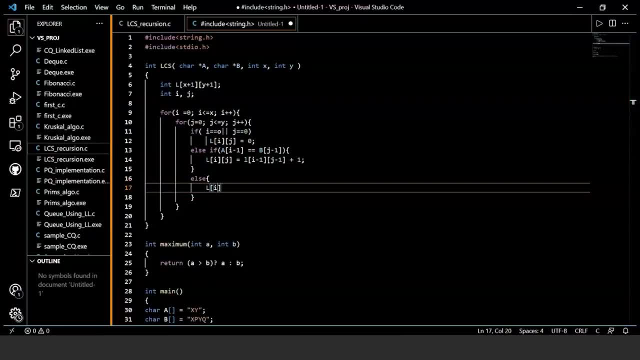 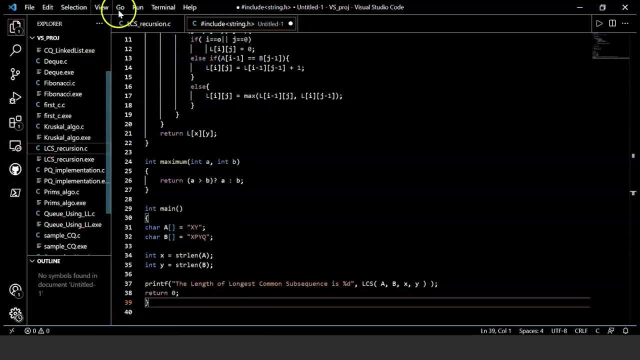 pick l ij as maximum of l i-large l, and here as well it should be large l, l, i-1, j-1 plus j comma, l i, j-1.. And we'll get out of these for loops and we'll return the output, that is, l, x and y. I hope this should be fine now. So let's run our code. 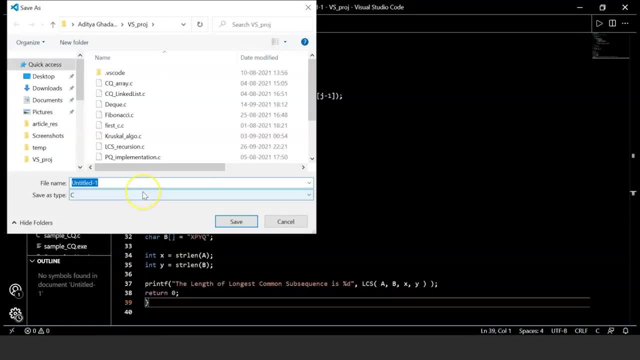 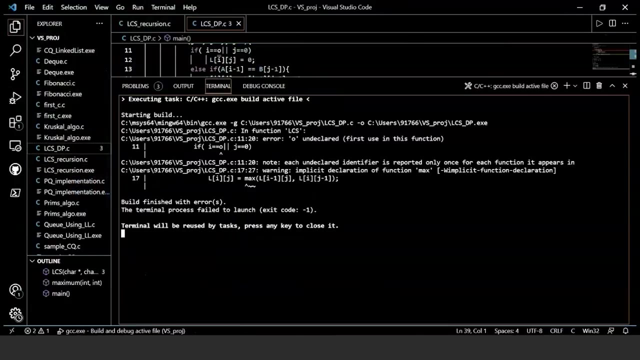 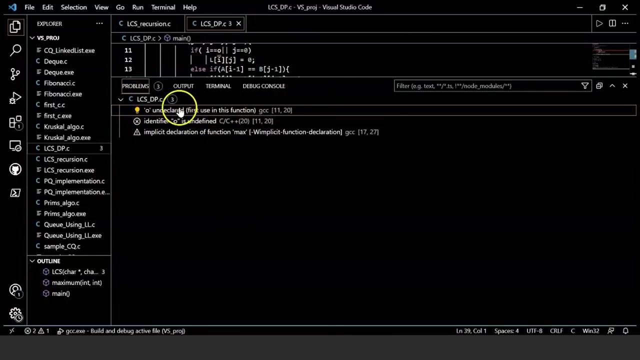 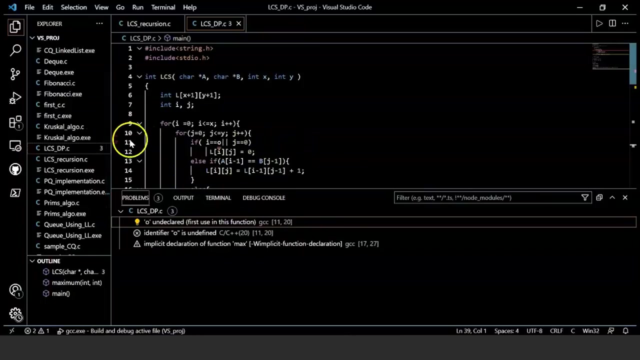 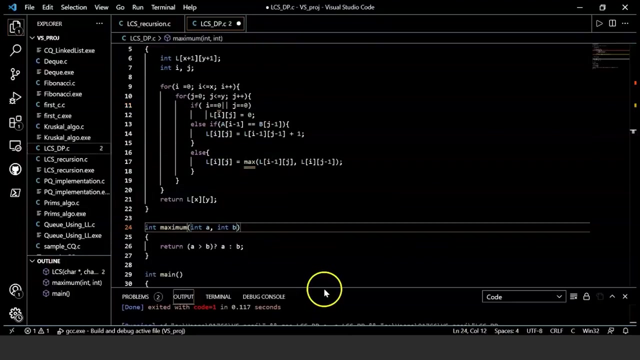 and check if there is something wrong. We'll save this as lcs. Okay, so we are getting three problems here. Okay, so I have inserted 4 here instead of 0.. And there is one more mistake. So I have called function max as max here and I have named 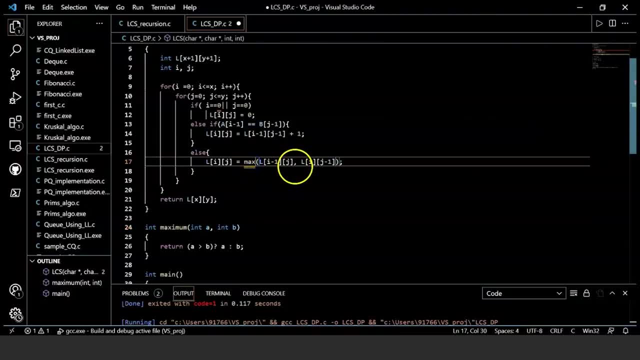 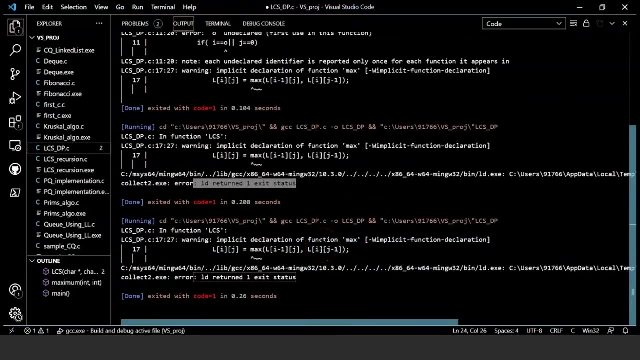 it as maximum here, So we'll have to change this to maximum. I think this should be fine now, So let's run our code again. Okay, we'll have to save this, Okay, Okay, Okay, I'll paste this. 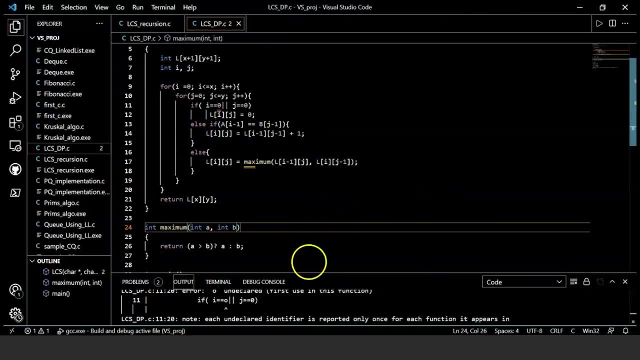 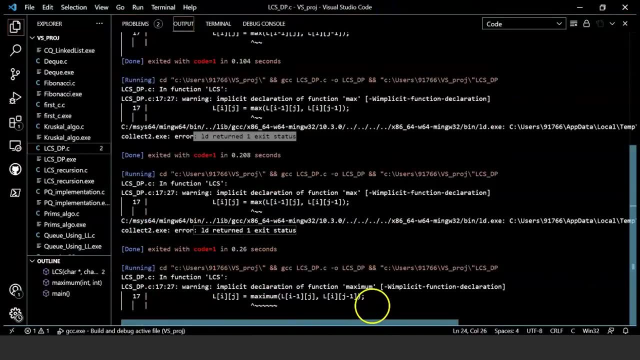 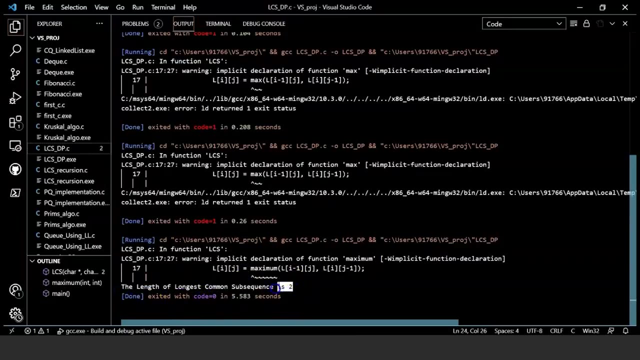 So we'll paste control s and we'll rerun it. Yeah, So we are getting our output here: the length of longest common subsequences 2.. So if you observe here the output that we have got using dynamic programming is in 5.58. 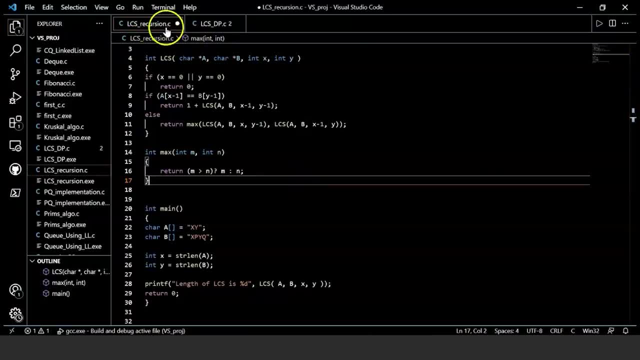 second And the time that was taken for LCS recursion was around 8 seconds. So you can see that the complexity has been reduced, The time complexity and space complexity as well. So that is why the dynamic programming is better approach than recursive programming paradigm. 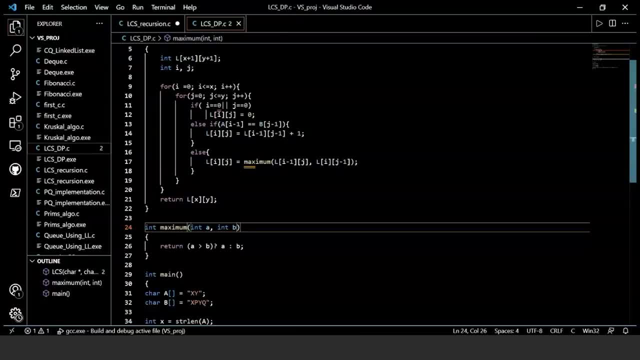 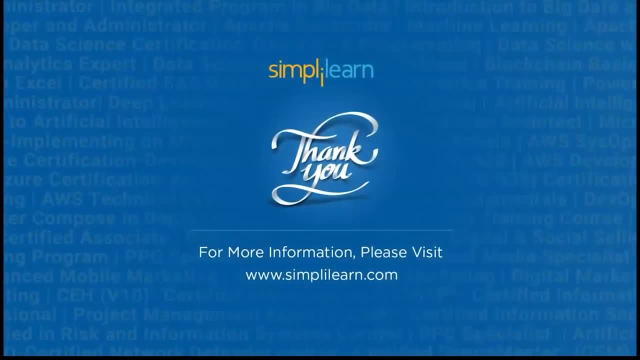 I hope the longest common subsequence problem- implementation using dynamic programming- is clear to all of you out there. So with this we came to the end of this video. I hope this video on longest common subsequence was informative. If you have any queries regarding this topic, then let us know about it in comment section below. 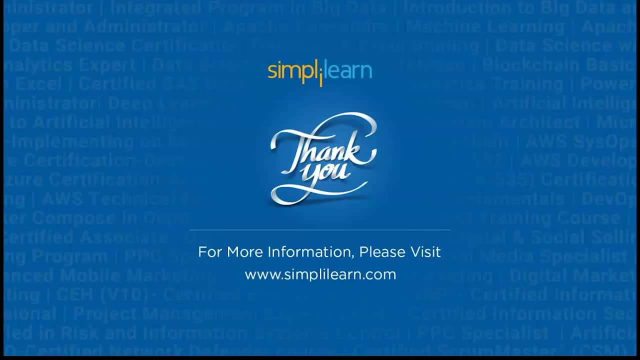 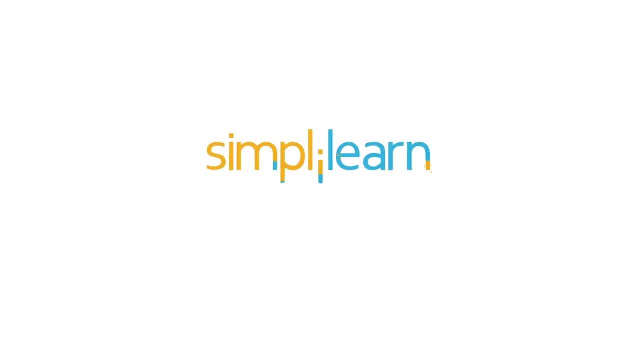 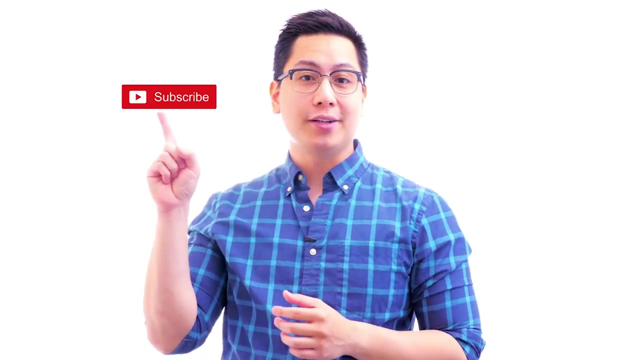 And we will get back to you. Thank you so much for being here and do watch out for more videos from us. Until then, keep learning and stay tuned to Simply Learn. If you like this video, subscribe to the Simply Learn YouTube channel and click here to watch similar videos.